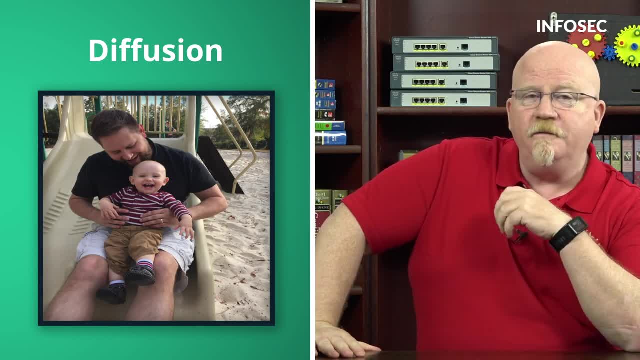 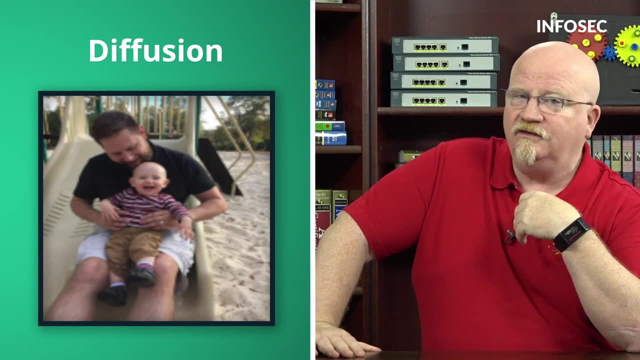 Let's take a look at that. That's Steven, Isn't he gorgeous? So what I'm going to do is I'm going to diffuse this image and make it fuzzier. Now, in this particular case, we didn't diffuse it too. 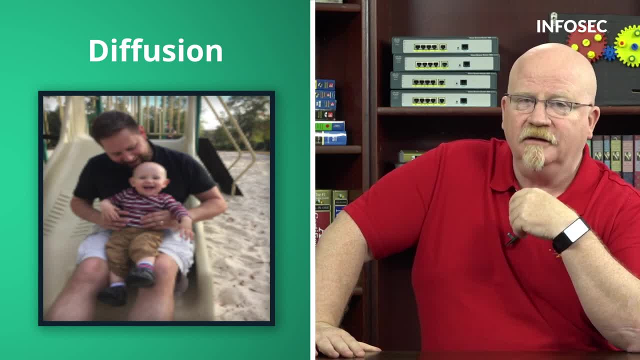 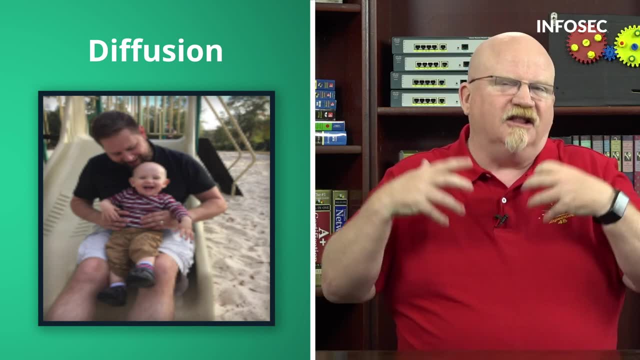 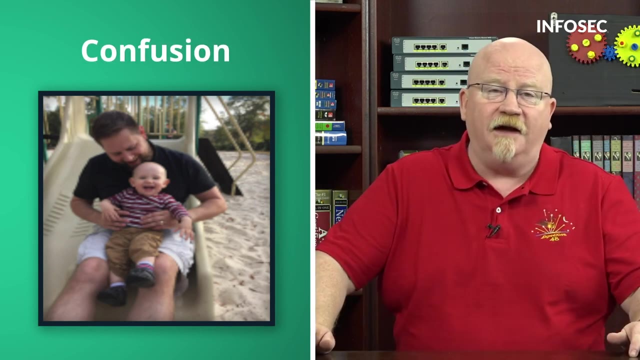 much So if you look at it, you could probably tell there's still a cute little kid there and he is cute. But diffusion only allows us to make it less visible, less obvious. Now, what we can also do is confusion. So let's take that same image of Steven one more time. 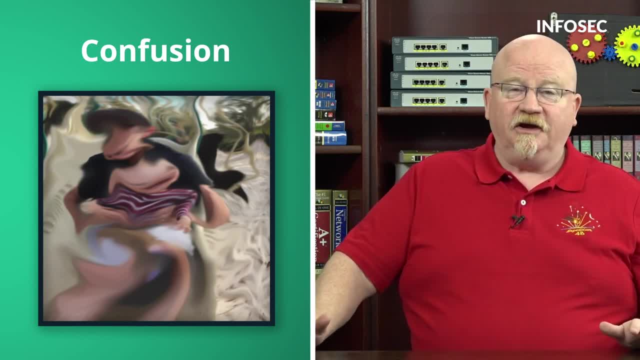 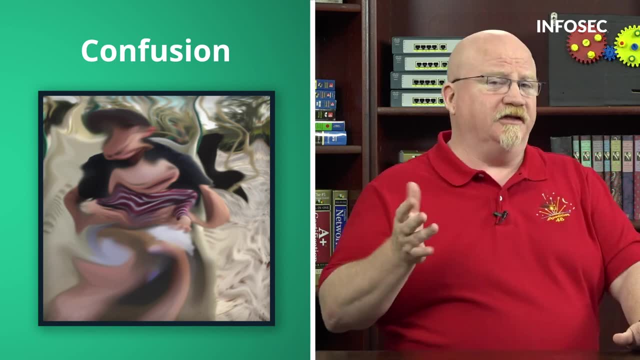 just stir it up. Let's just make a mess out of it. Now, in this particular case, we've created a lot of confusion of the image. It's basically stirred up and it would be very difficult for somebody to simply look at this and go, ah, that must be Mike's grandson Steven. So the other challenge we have 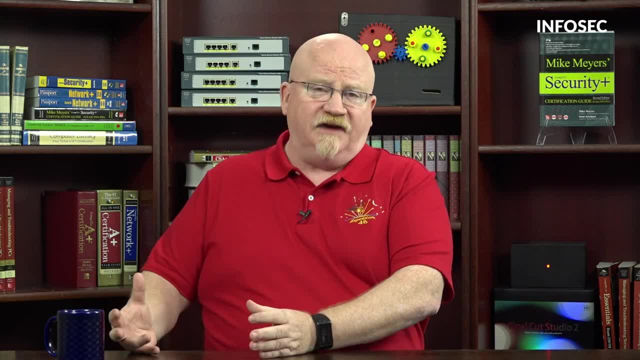 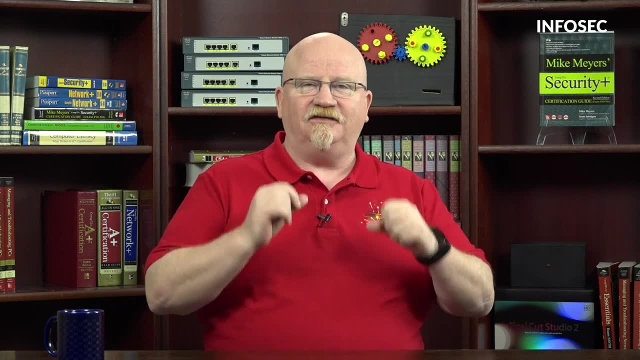 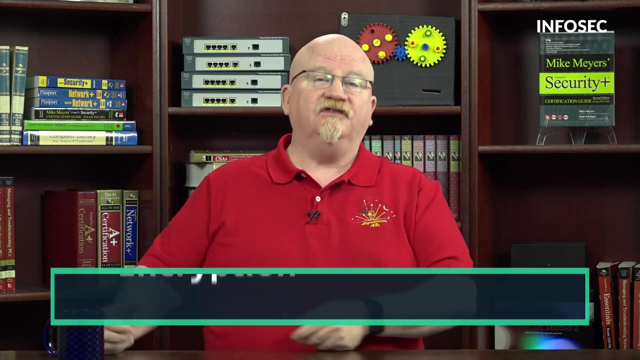 with cryptography is we go through this process of taking some kind of data and we go through this process of taking some kind of data and we go through this process of taking some kind of data and some way bring it back into its original form. So we call this encryption and decryption. 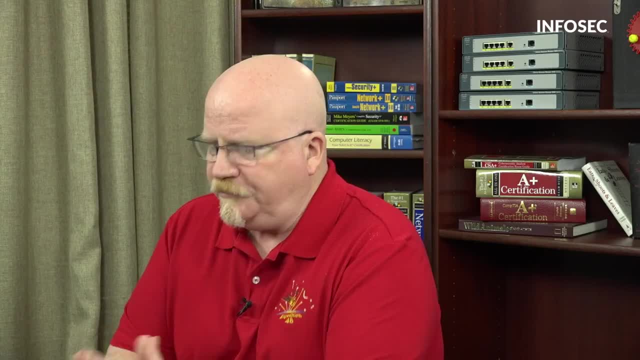 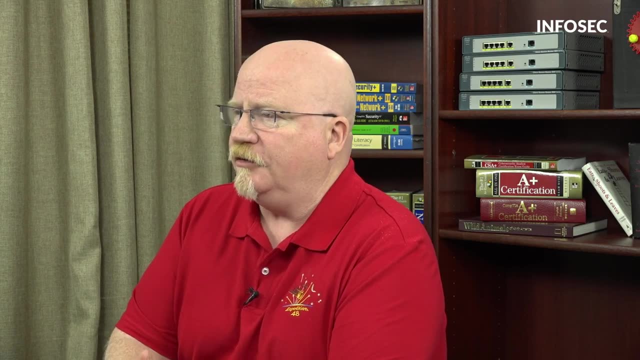 And cryptography is the process of making this happen. Cryptography has been around for a long, long time. In fact, probably one of the oldest type of cryptography has ever been around is something called the Caesar cipher. I don't know about you, but when I was a little kid- 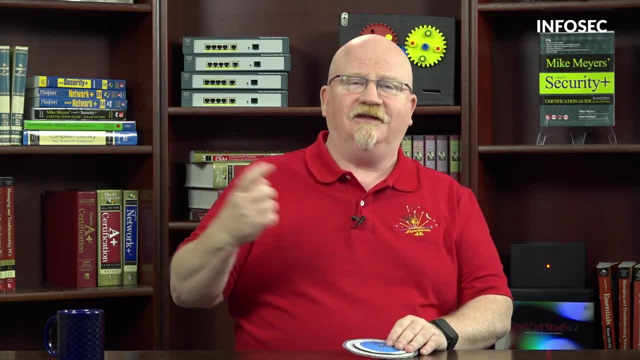 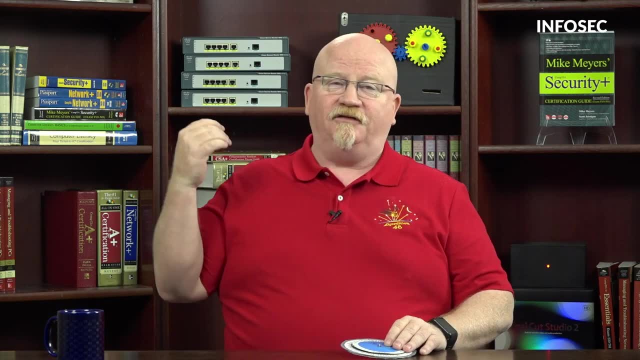 and I was eating a box of cereal. I was eating a box of cereal and I was eating a box of cereal. you'd dump out the box of cereal and you'd get some kind of prize inside, And one of the things we'd get is called a secret decoder ring. So what I want to do here, let's can we put up a picture? 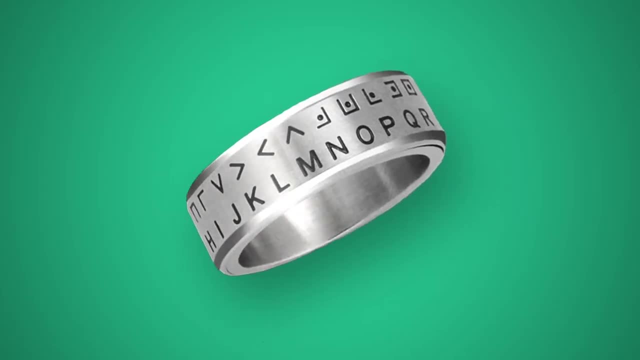 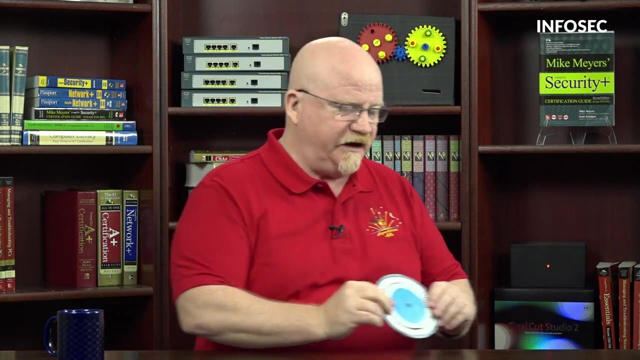 of a secret decoder ring real quick. Okay, so this is a classic old school kids decoder ring. Now what I want to do is I've made my own decoder ring right here and I'd like us to take a little peek at this guy. And what you're going to see here is I basically got a wheel with all the 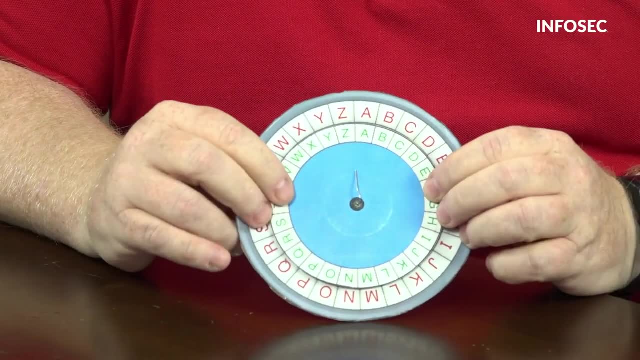 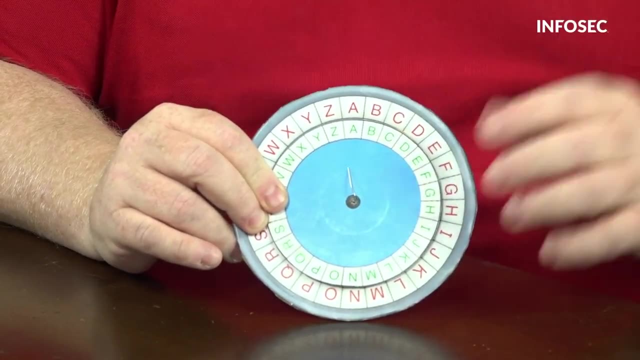 letters of the alphabet A through Z, and on the inside I've got letters of the alphabet A through Z. So right now I've got them lined up: A to A, B to B, C to C. Now what I can do to make a secret. 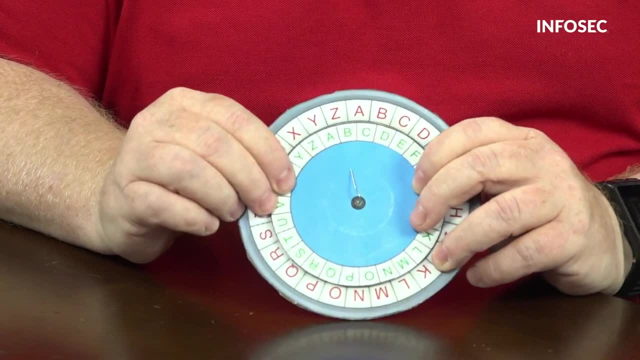 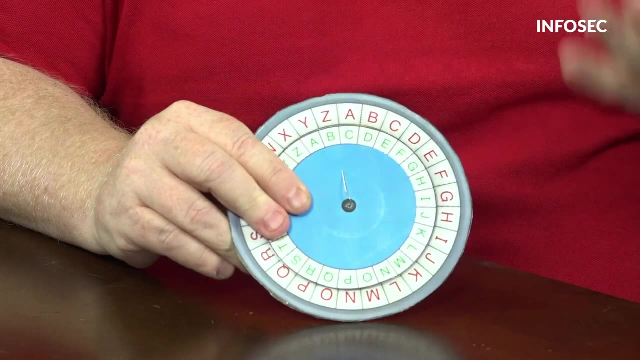 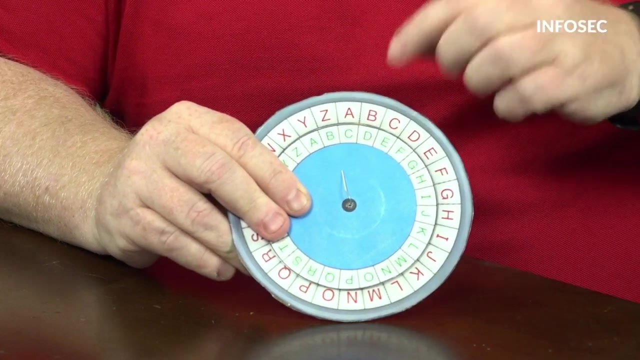 code is: let's say, I can turn this two, I can rotate this two times, And what we can do is we can take our original plain information, what we call the plain text, our message that we want to encrypt, and we just change the letters. So we call this substitution What we'll 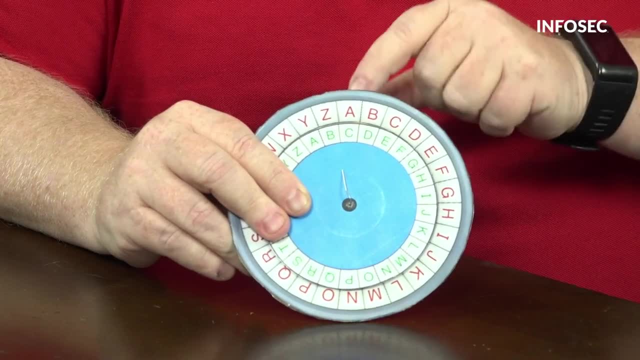 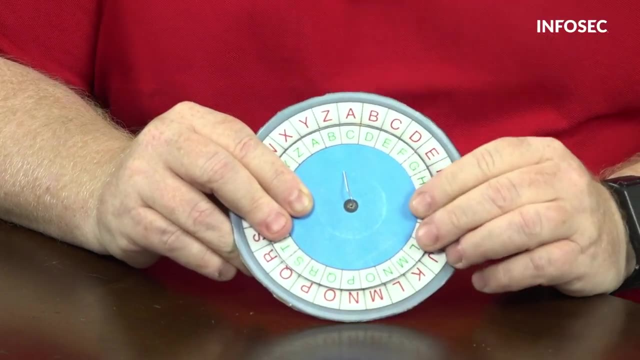 do is we'll take one value and substitute it for another. Now, in this case, I've rotated it twice, so we actually have a term for this. We call it R-O-T-2, just like that. And if I turned it, 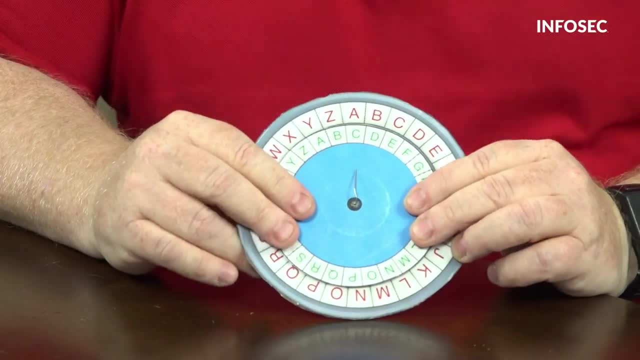 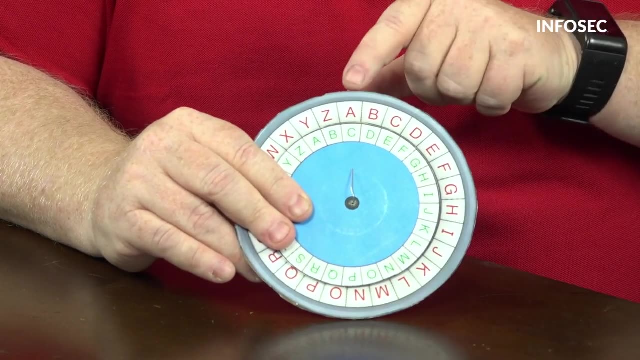 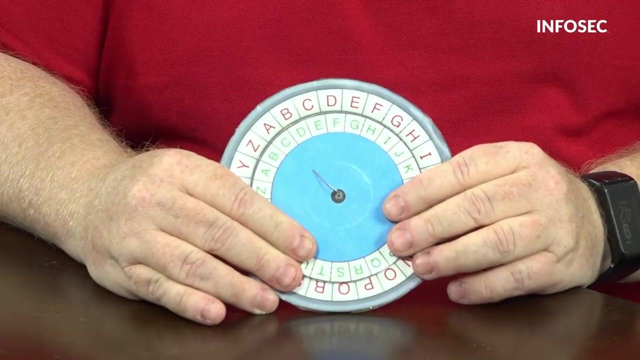 three times it would be R-O-T-3.. Now, so we can take like the word ACE, A-C-E, and I can change A-C-E to C-E-G. Get the idea. So that's the cornerstone of the Caesar cipher. So to convert, 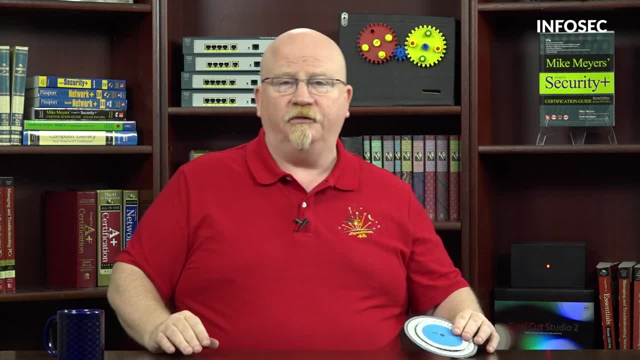 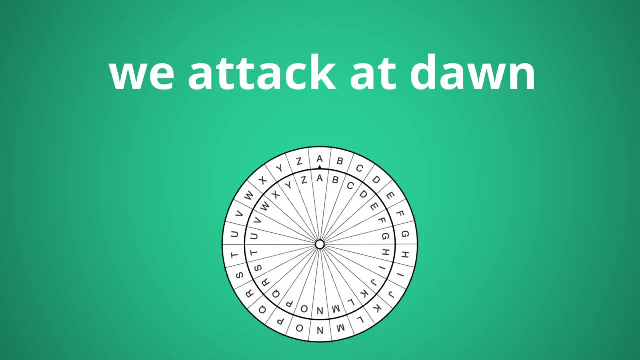 something with the Caesar cipher and, as a matter of fact, let's just go through the process real quick. Now what I'm going to do: let's put up a piece of plain text that we want to encrypt. We attack at dawn. So here it is: we attack at dawn. Now, the first thing we're going to do: 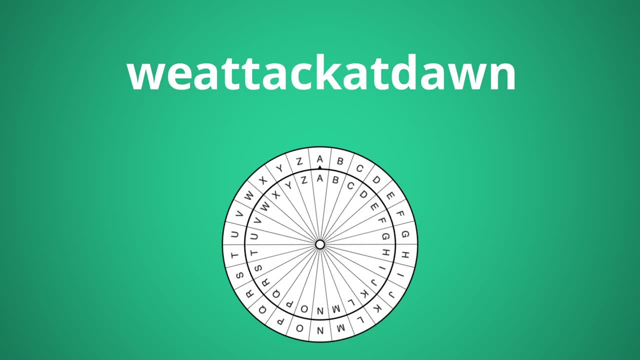 get rid of all the spaces. So now it just says: we attack at dawn, very readable. We don't worry about upper or lower case in this particular situation. Now let's go ahead and put our groovy little secret decoder ring up there And let's go ahead and turn it in this particular 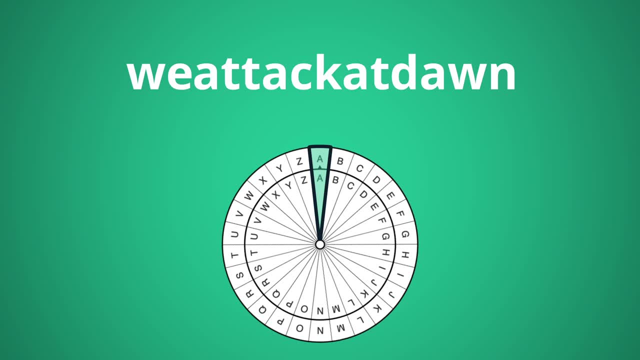 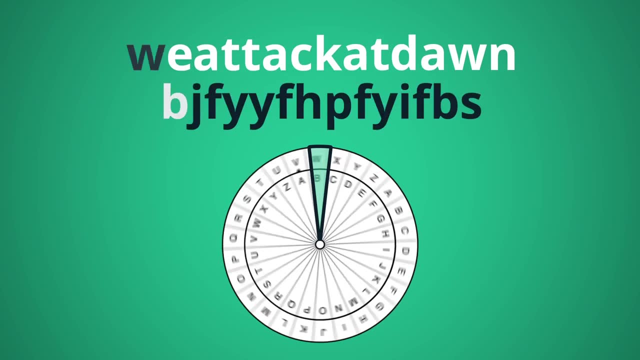 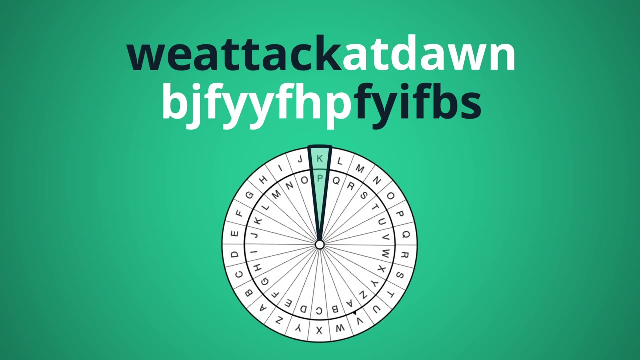 case five times. All right, So we're doing an R-O-T-5.. So let's turn it one, two, three, four, five times. So now what we can do is, by using the secret decoder ring, we can go ahead and encrypt. We attack at dawn as follows. So what we now have generated: 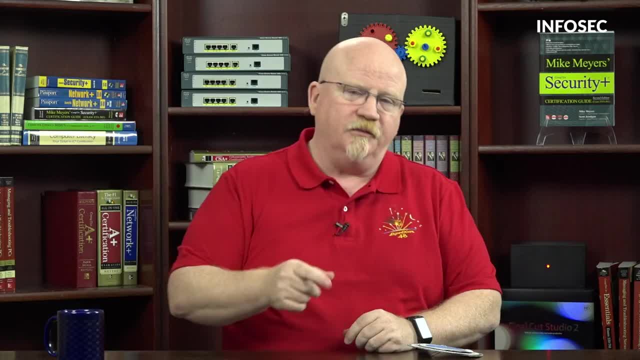 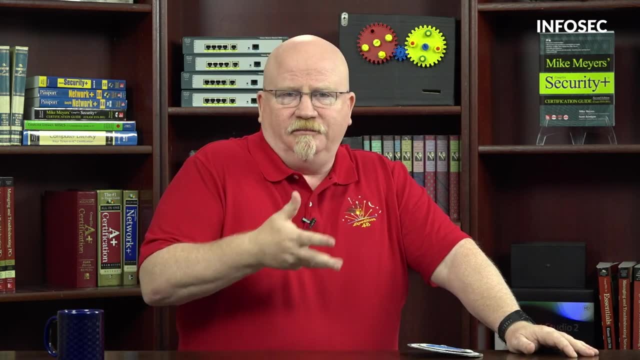 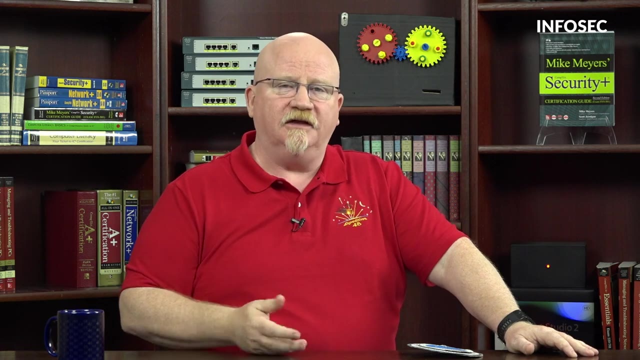 is a classic Caesar cipher. Now, there's a problem with Caesar ciphers, And the biggest problem we have with them, more than anything else, is that, in fact, people who buy crossword puzzle books will pay money to be able to do this is that we can decrypt them. We can just by looking at them. 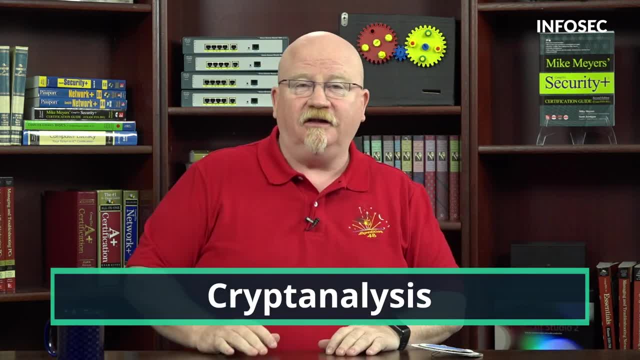 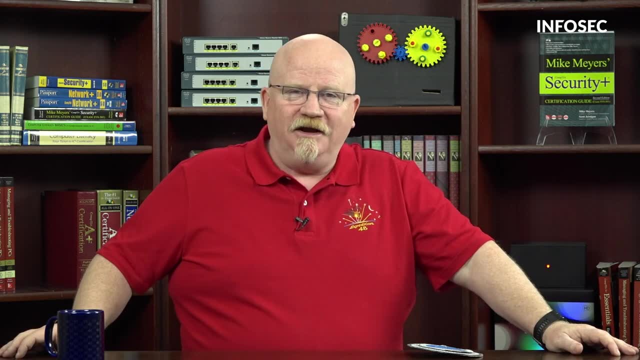 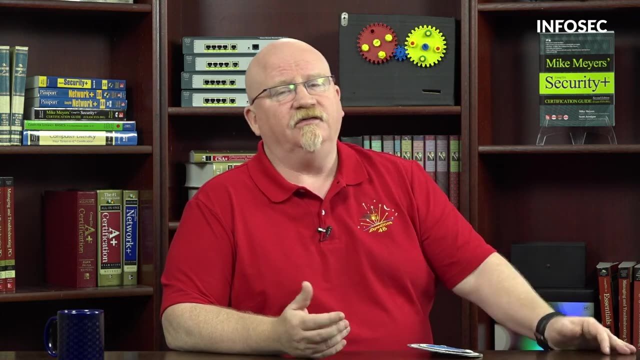 we can provide what's known as cryptanalysis. Cryptanalysis is breaking these encrypted codes, So the problem is is that anybody who's good at these things could pretty easily crack this. So the Caesar cipher, even though it is a substitution cipher, does have. the problem is that it's just 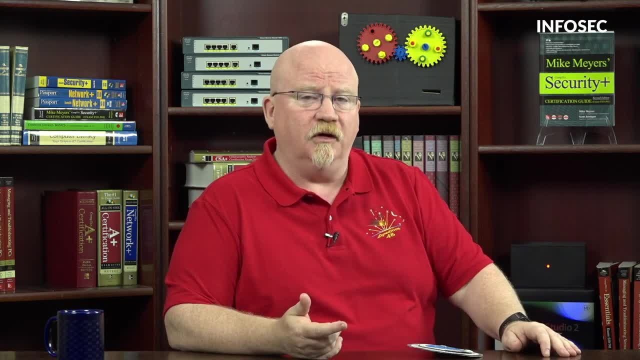 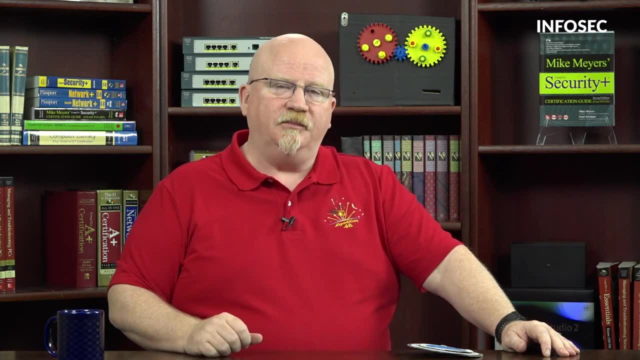 too easy to predict what's going to happen, So we're going to do a little bit of a decryption. I'm going to show you what this is, because we're used to looking at words, So what I want to do is make it a little bit more challenging. The first thing I'd like to try to do is I want to bring in 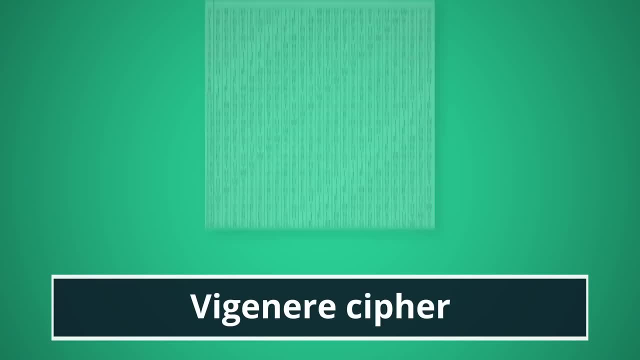 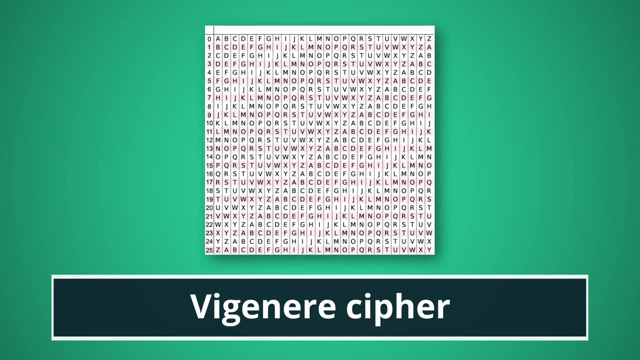 something called the Vigenet cipher. The cornerstone of Vigenet cipher is that it's really just a Caesar cipher with a little bit of extra confusion involved. So what I've got here is a table that shows all the possible Caesar ciphers there are. So here up at the top, we're going to have the 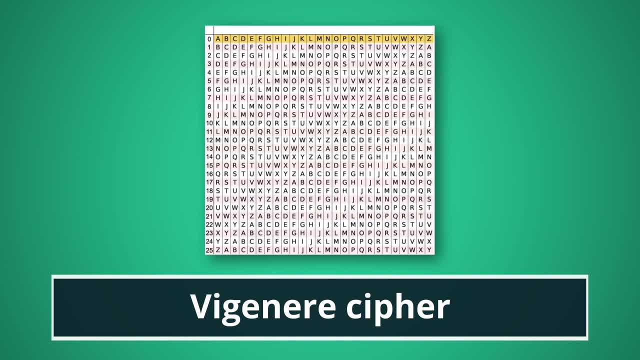 word plain text. I'll show you how that works And then we're going to have a little bit of a look at how that works in just a minute, And then you'll see on the far left hand side it says zero through 25.. So these are all the possible ROT values you can have from ROT zero, which means 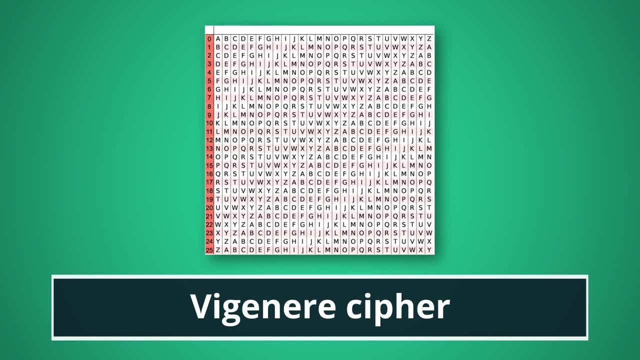 A equals A, B equals B, all the way down to ROT 25.. So what we're going to do, let's hold on to this for a minute, And now let's go ahead and start with a piece of plain text Let's use. we attack at. 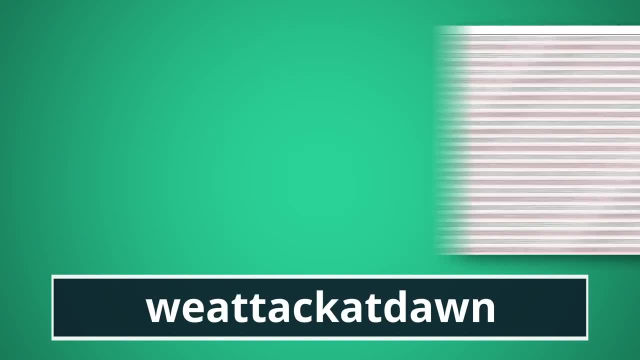 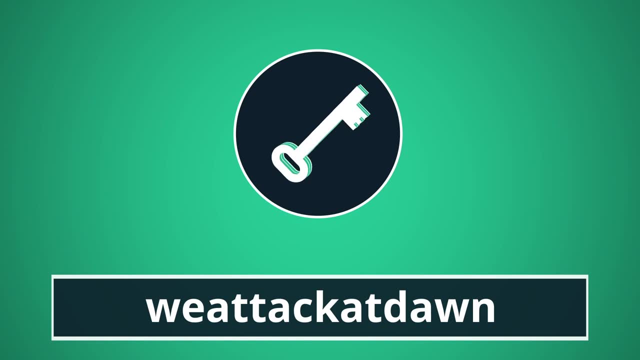 dawn one more time, And what I'm going to do this time is we're going to apply a key. The key is simply a word that's going to help us do this encryption. In this particular case, I'm going to use the word face, F-A-C-E. Now, what I'm going to do is I'm going to put F-A-C-E above the first. 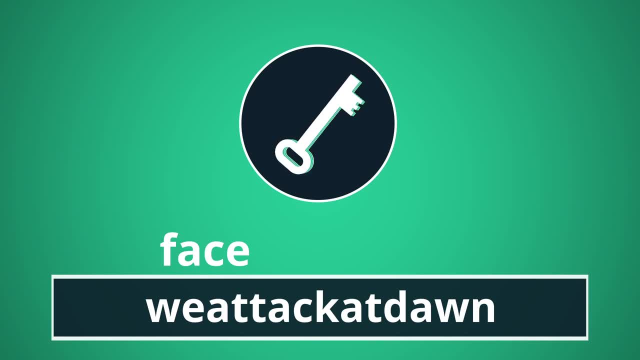 four letters of: we attack at dawn. So here we go, F-A-C-E, And then I'm going to just keep repeating that. So let me put face again. I'm going to put face again And you'll see, I've got two letters. 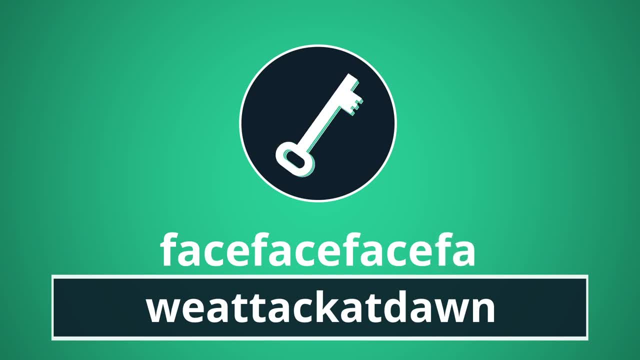 left over. No big deal. I'll just put F-A, And what we've done is we have applied a key to the plain text. Now what we're going to do is we're going to use the key to change the Caesar cipher ROT value for every single letter. So let's go ahead and do this. Now, what I'm going to do is: 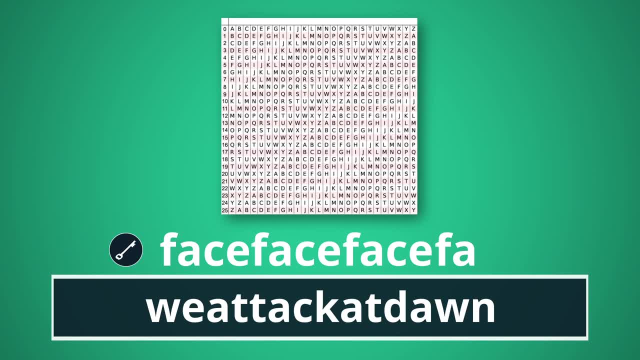 I'm going to reference my little chart here. So the first letter of the plain text is the W in we. So here's the W up at the top, And the key value is F. So let's go down on the y-axis. 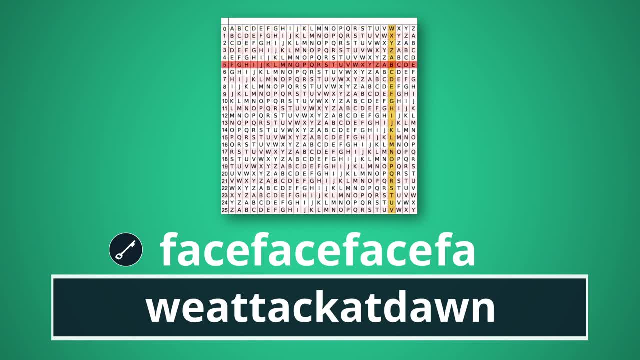 Here until we get to an F. Now you see that F. you'll see the number five right next to it. So this is ROT five. So all I need to do is do the intersection of these and we get the letter B. Great, Let's do it again Now. in this case, the second time it's the letter E from we, And in: 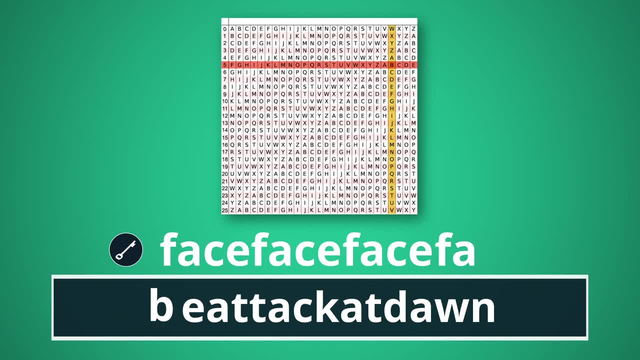 this particular case, the key value is A, which is kind of interesting because that's ROT zero, but that still works. So we start up at the top, find the letter E, Then we find the A And in this case it's going to be zero. by coincidence, E is going to stay as E. Let's do the third value. 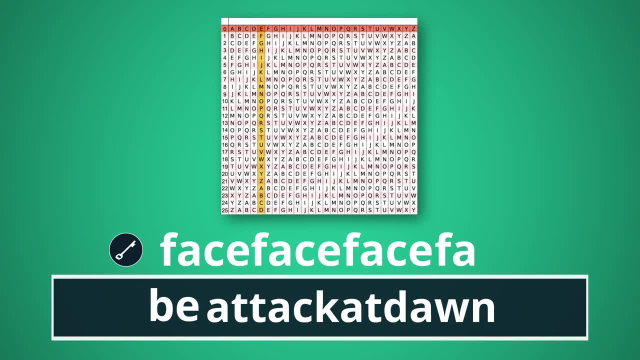 Now, this time it's the A, as in attack. So we go up to the top, There's the letter A And the key value is C, as in Charlie. So we go down to the C, That's ROT two, And we then see that the letter A. 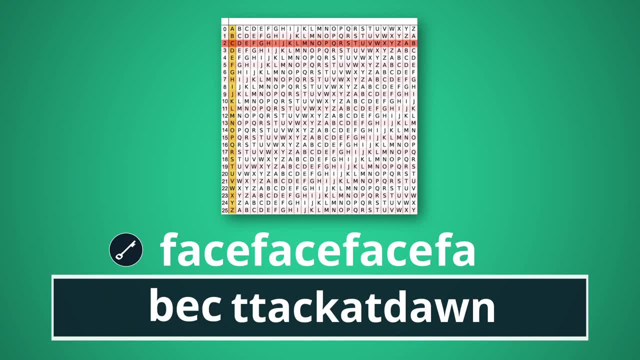 is now going to be C. Okay, let's do one more real quick. In this particular case, it's the first T to the T's And now the key value is E, as in face. So we go down here. That's ROT four. We do the. 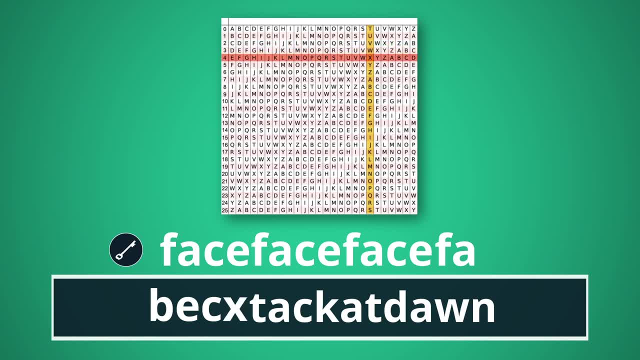 intersection. And now we've got an X. So the first four letters of our encrypted code is BECX. So let's go ahead and run through and do the rest of these real quick. I'll just put those in for you. And we have now encrypted in the Vision A style. So the beauty of the Vision A is that it. 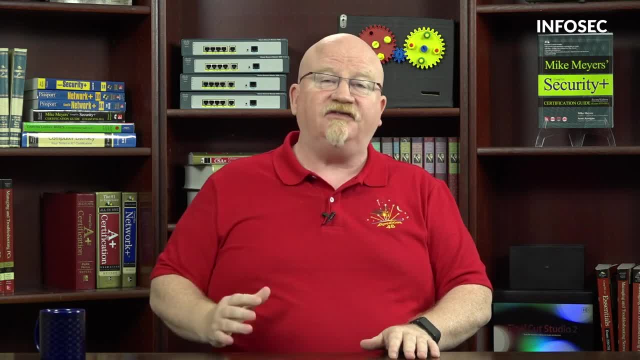 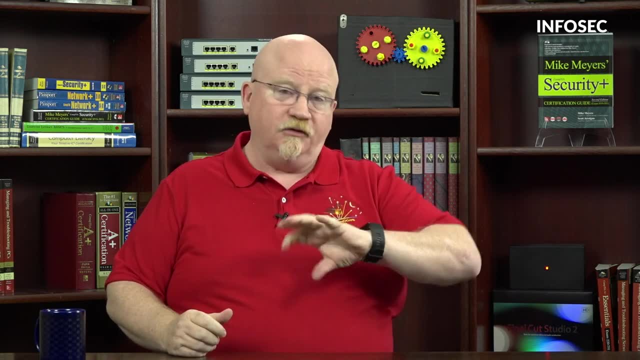 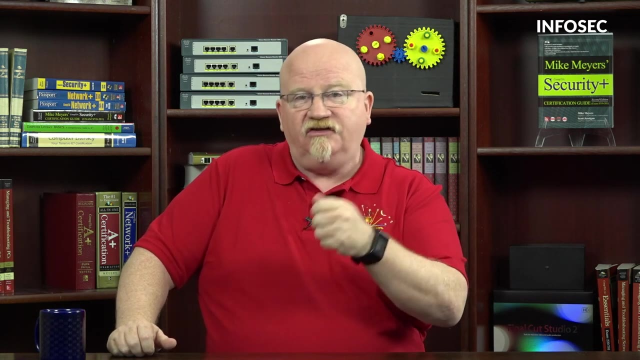 gives us all the pieces we need to create a classic piece of cryptography. Number one: we have an algorithm, And the algorithm are the different types of Caesar ciphers and the rotations. And second, we have a key, And the key allows us to make any type of changes we want within ROT zero. 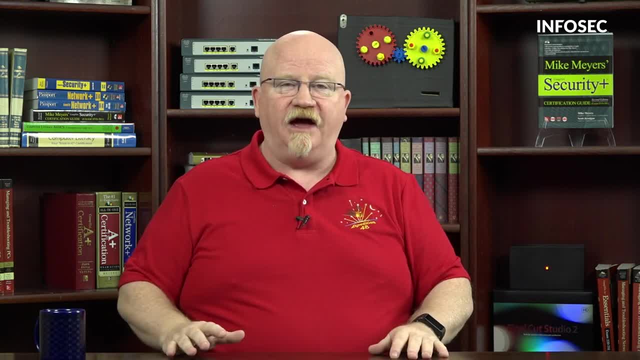 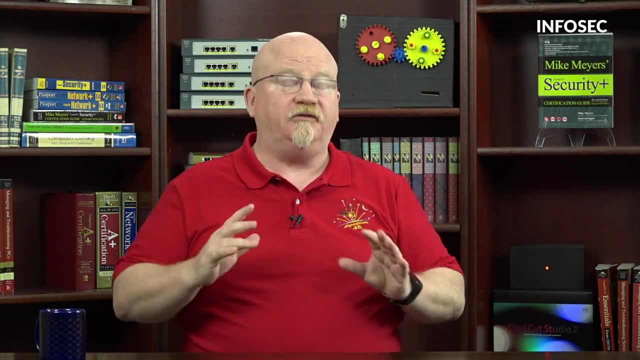 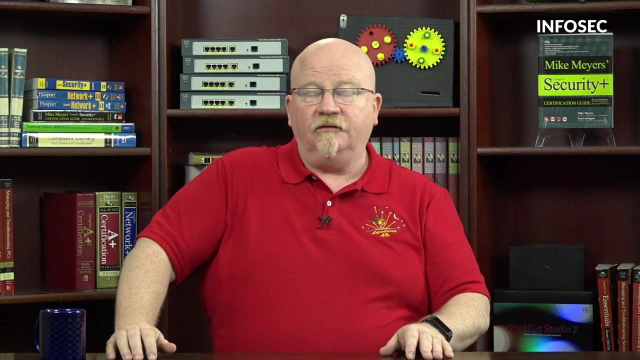 to ROT 25 to be able to encrypt our values. Any algorithm out there is going to use a key in today's world. Now we'll be talking about cryptography. Today, We're always going to be talking about algorithms and keys. Now, the problem with the Vision A is that. well, number one, it's surprisingly crackable. 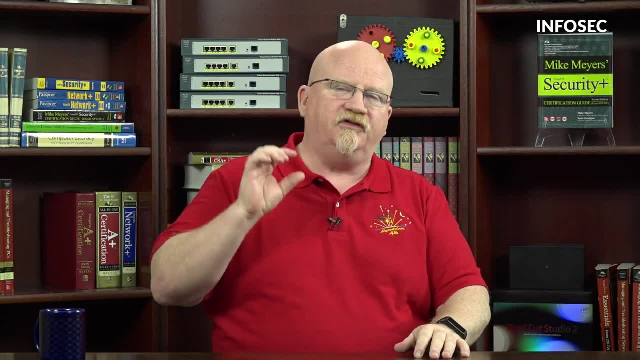 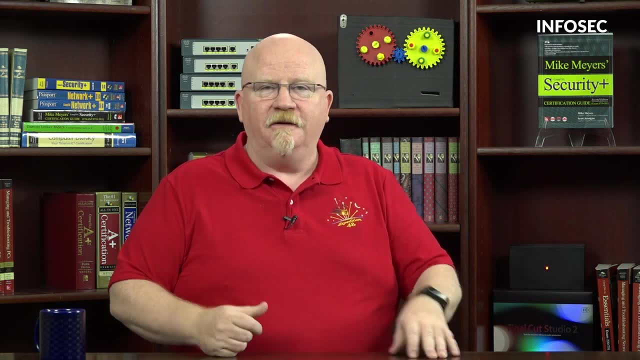 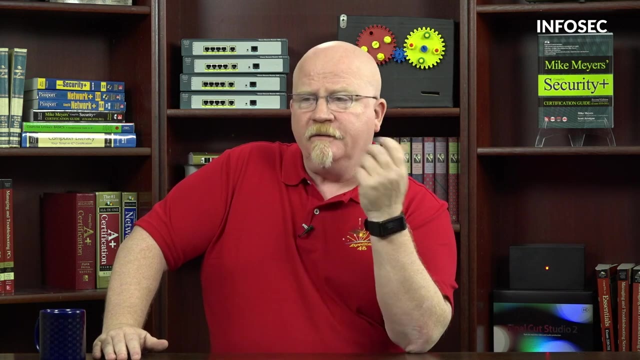 Isn't that interesting. But the bigger problem this is vision a works just great for letters of the alphabet. Unfortunately it's terrible for encrypting pictures or SQL databases or your credit card information. In the computer world, everything is binary, everything is binary. 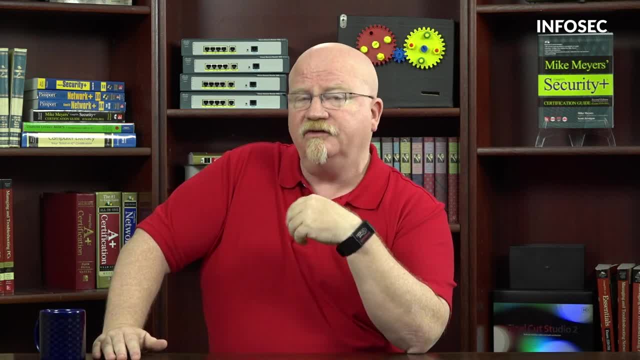 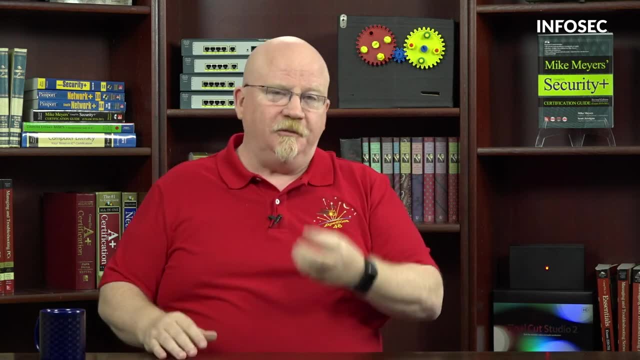 As a smart devicefsxac In the data science world. just the non forensic Judaism school thinks one of the worst Turkish madem� is ones and zeros. So what we need to do is come up with algorithms that provide the type of encryptions and decryptions we need. 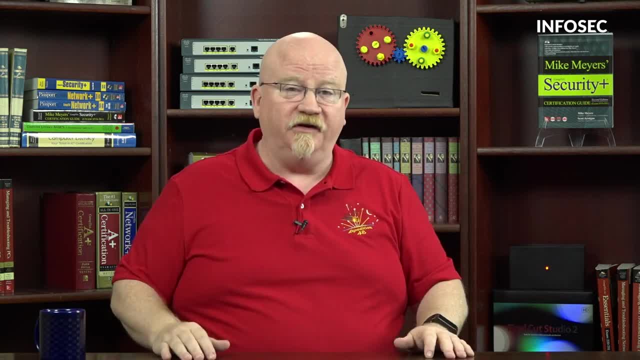 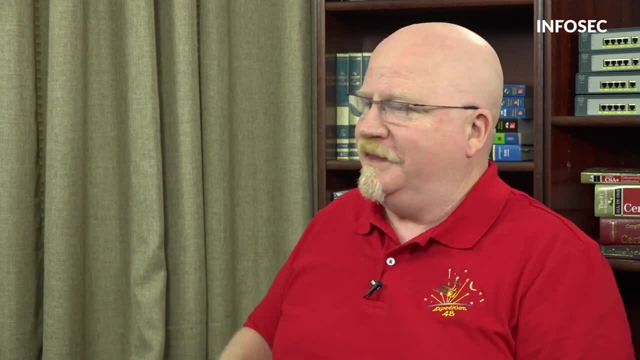 to encrypt and decrypt long strings of just ones and zeros. Now, if you look at a string of ones and zeros, you go: how does anybody make anything out of this? Well, they do. You got a string of ones and zeros. may look like nothing to you, to a human being. 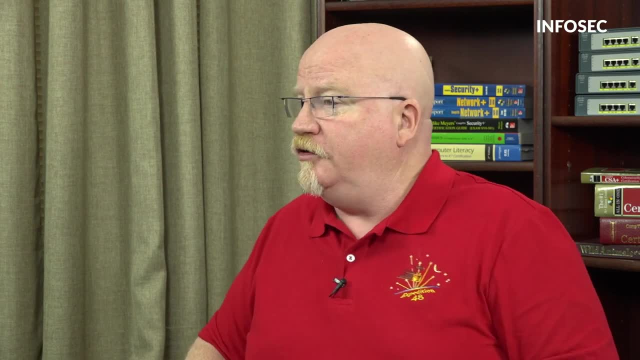 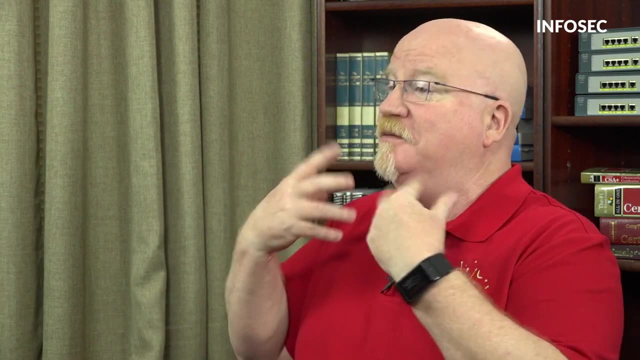 but to Microsoft Word. that could be a Word document, Or it could be a voice over IP conversation, Or it could be a database stored on a hard drive, I don't know. but just because as human beings, we look at long strings of ones and zeros and get confused, 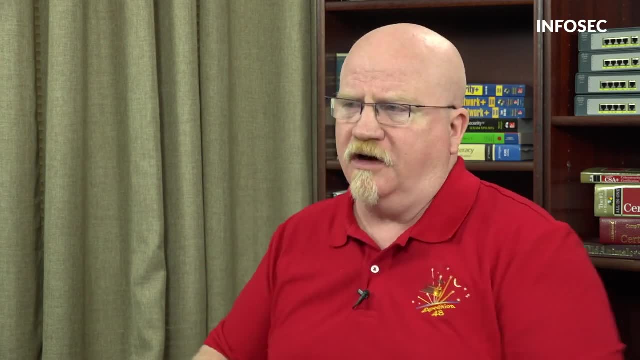 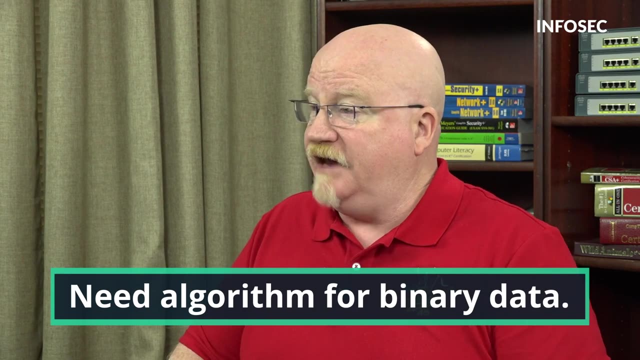 Trust me, the computers don't. What we need to do, though, is we need to come up with algorithms which, unlike Caesars or Vision A's that will work with binary data. Now, luckily for us, there are a lot of different ways. 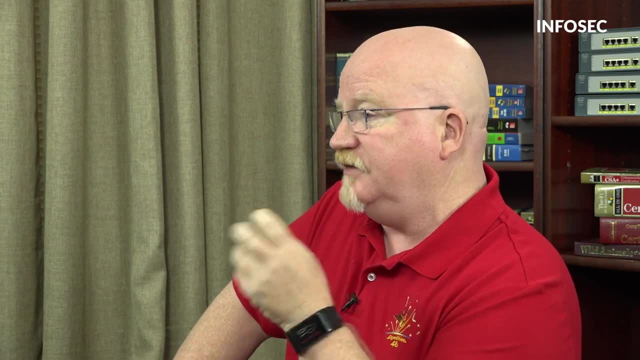 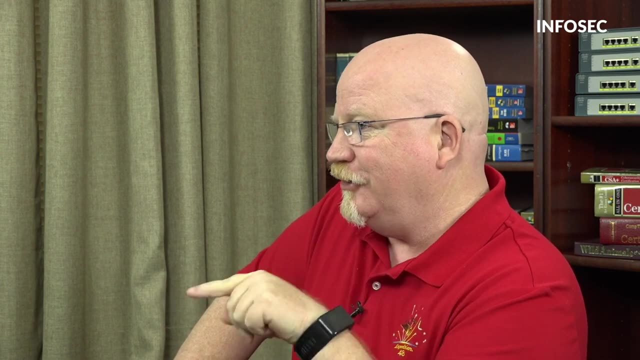 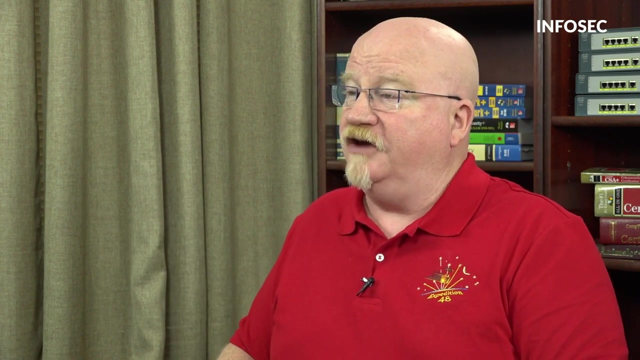 to do this. So what we're gonna do is- I've got an example of a algorithm we're going to use that encrypts a simple phrase, that we're gonna convert those to binary, by the way, and we're gonna do this using a very interesting type of binary calculation. 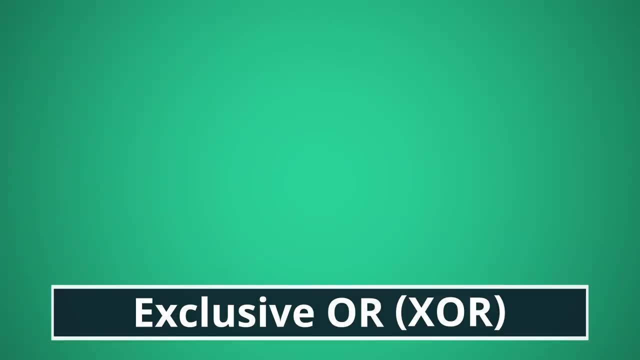 called Exclusivore, For our first encryption. I'm going to encrypt my name, So here's my name: Mike M-I-K-E. Now, the first thing we're gonna have to do is we're gonna have to convert this to the binary. 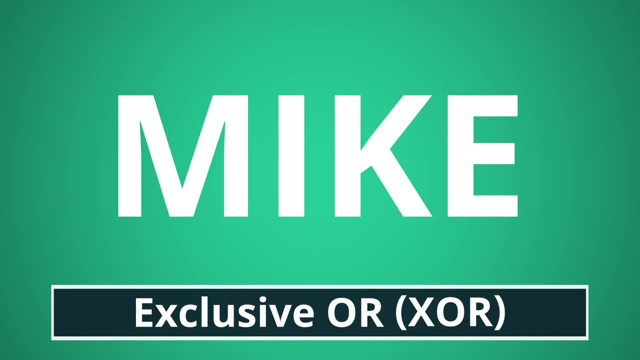 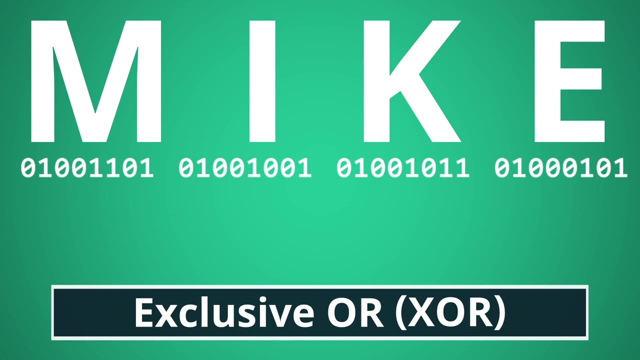 that a computer would use. So I'm going to be using the binary equivalence of these text values. So let me go ahead and convert these into their binary equivalents, And anybody who's ever looked at ASCII code or Unicode should be aware that we can convert these into binary. 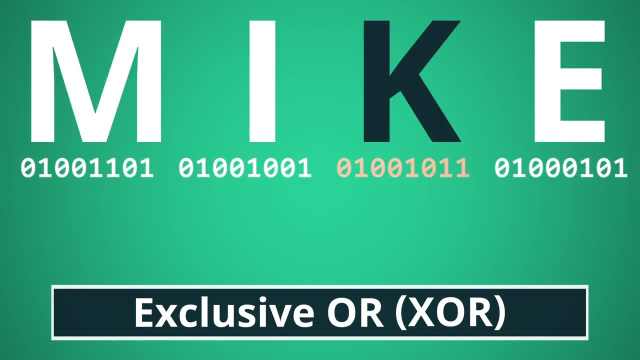 Okay, so here we go. So here's M-I-K-E converted into binary. Now notice that each character takes eight binary digits. So we've got 32 bits of data that we need to encrypt. So that's our clear text. Now, in order to do this, we're gonna need two things. 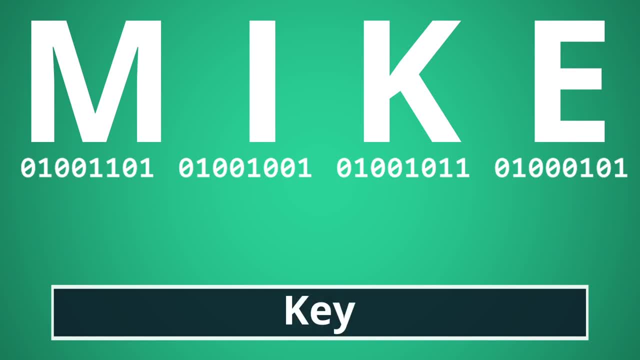 First of all, we're gonna need an algorithm, and then we're gonna need a key. Now keep in mind, what I'm making up is like the most simple version of encryption you can possibly do. So let's go ahead and first of all, set up our algorithm. 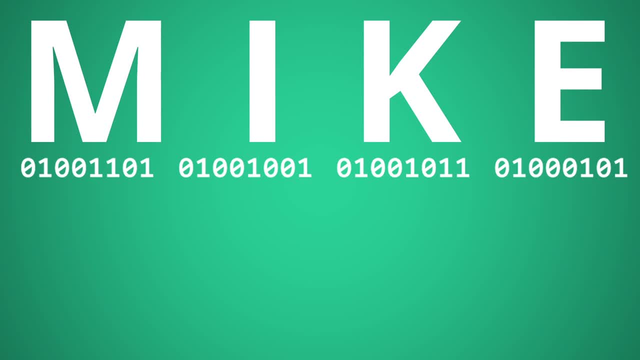 Now, our algorithm is extremely simple, using what we call an Exclusivore. So here's the Exclusivore. This is what we call a truth table. So what I'm gonna do is I'm gonna choose, because this Mike algorithm arbitrarily chooses this. 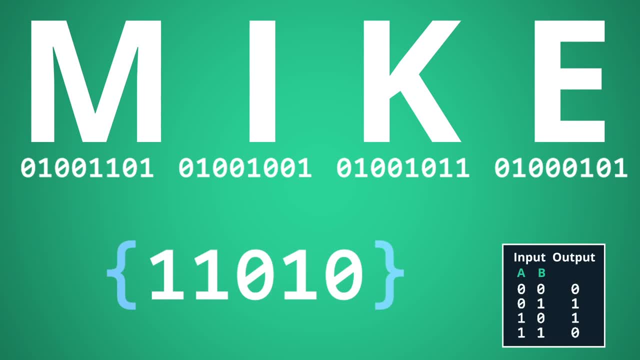 is, I'm going to be using a five-bit key. Now there's a reason I'm using a tiny, tiny, short key like this. In the real world, keys can be thousands of bytes long, But for right now we're just gonna use a five-bit key. 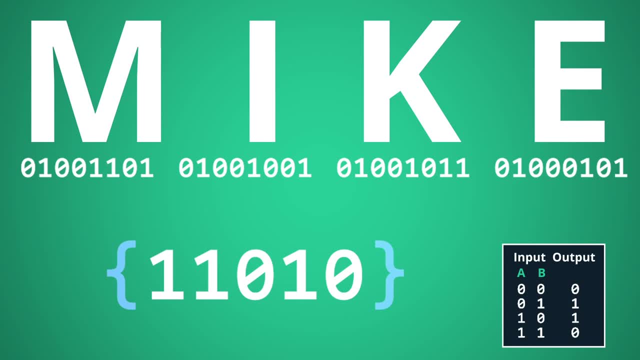 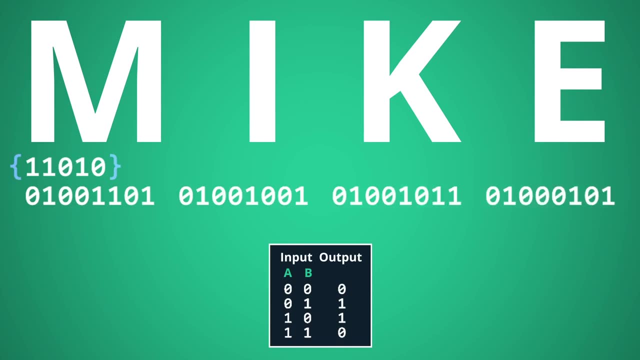 So to make this work, let's start placing the key. So I'm gonna put the key over the first five bits. So here at the letter M for Mike, And now we can look at this table and we can start doing the conversion. 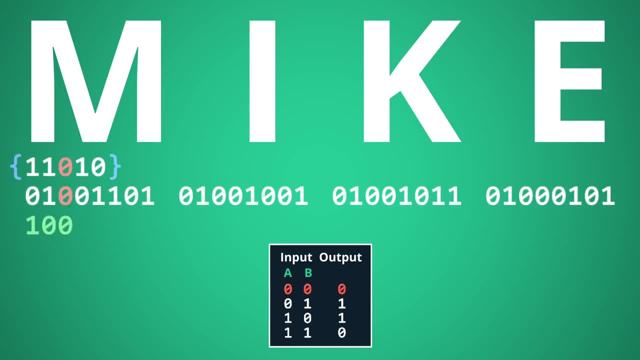 So let's convert those first two values, then the next, Then the next, Then the next. Okay, so now we've converted a whole key's worth, But in order to keep going, all we have to do is schlep that key right back up there. 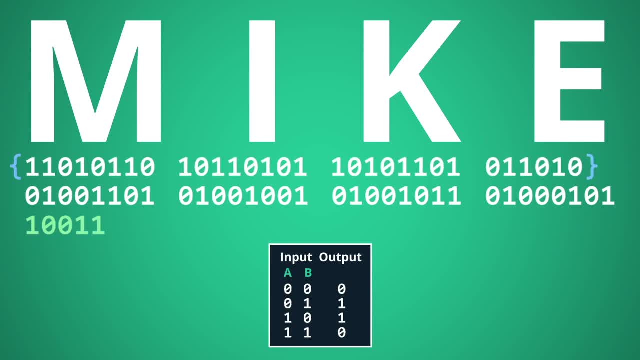 Okay, In fact, let's go ahead and extend the key all the way out: Boop, boop, boop, boop, boop. So now the key. we just keep repeating it And you'll see here at the end it doesn't quite line up. 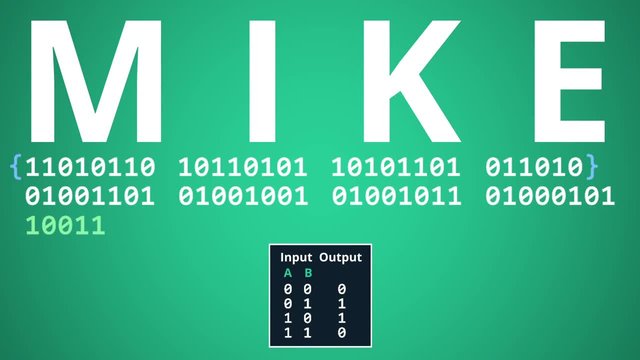 No problem, Just add whatever amount of key you need to go ahead and fill up the rest of this. So there we go. Okay, So now we can go ahead and complete this. Now, let's just do it fast. You can double check me if you want. 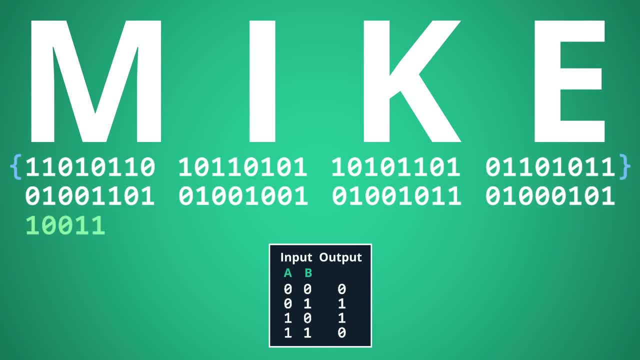 But as we go through here using the exclusive OR algorithm, we then create our cipher text. Go ahead and spot check a couple of those for me and make sure I got them right. Okay, beautiful Now. so this is the cipher text.